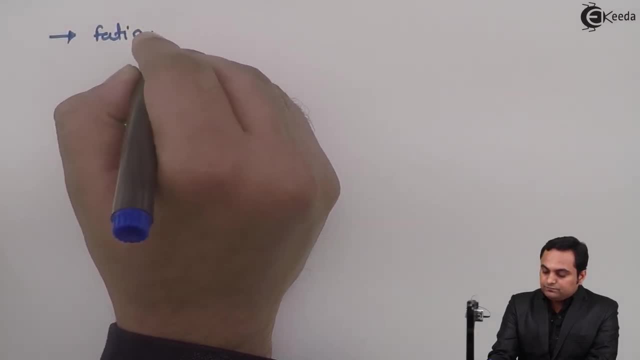 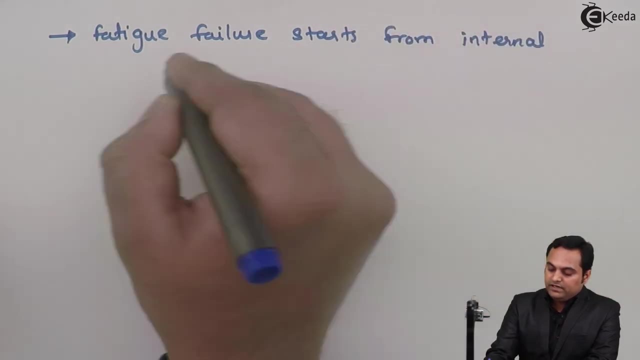 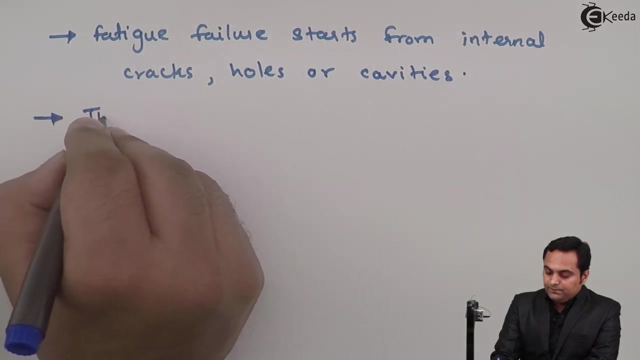 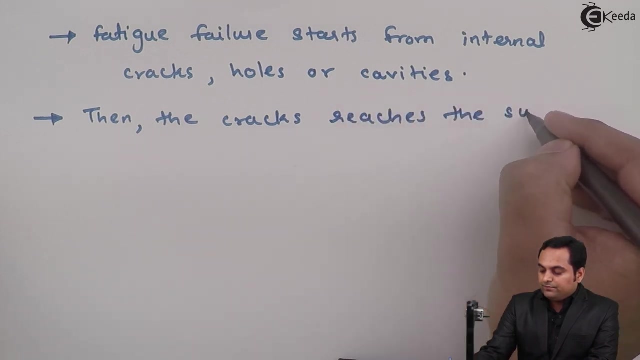 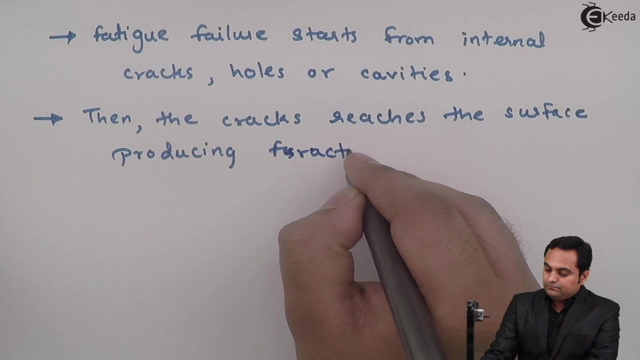 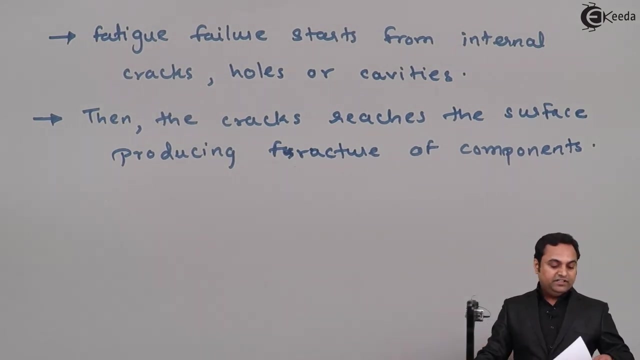 site. Next, I will add here: fatigue failure starts from internal cracks, holes or cavities. Then the cracks reaches the surface, producing fracture of components. So these are some points related to fatigue failure. Next, I can say that in case of fatigue, the stresses may be tensile or compressive, and 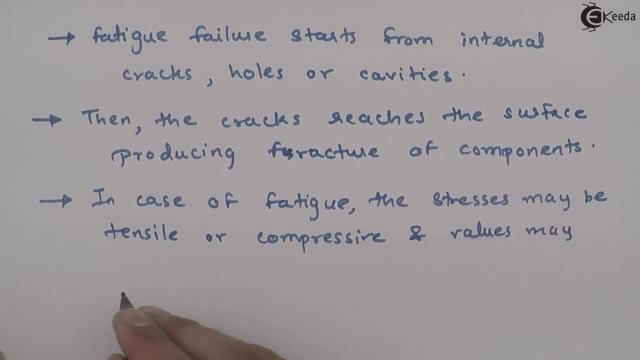 values may range from minimum to maximum. Next, I can say that, in case of fatigue, the stresses may be tensile or compressive, and values may range from minimum to maximum. That is, for fatigue to take place, the stresses can change from tensile to compressive or 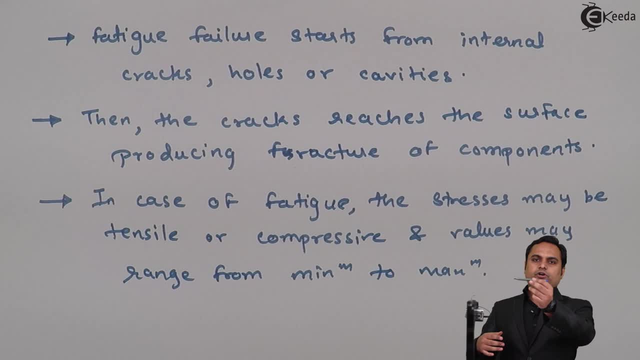 minimum to maximum values. Like, for example, if we have a rod and I want to break this rod, then I would be twisting this rod and then untwisting it, twisting and then again untwisting. So because of this continuous action the material will break and such kind of failure. 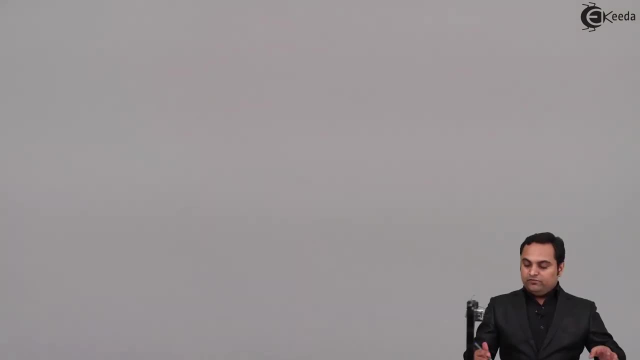 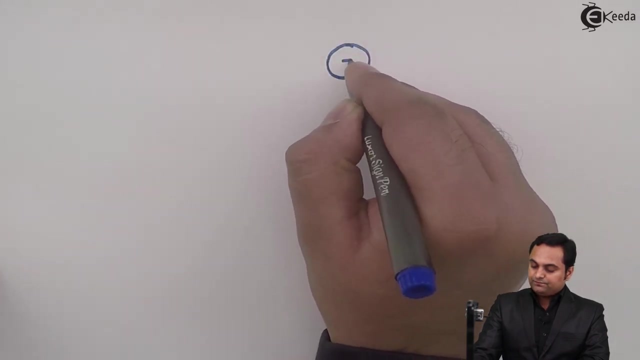 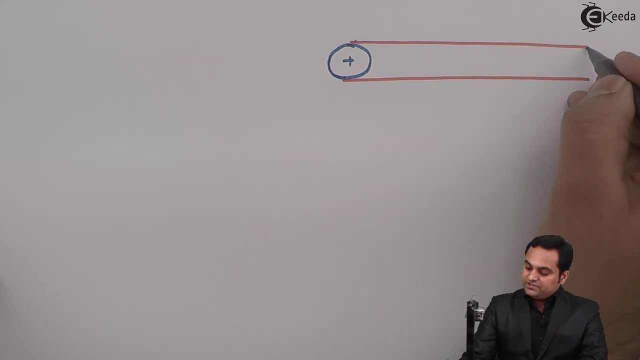 is called as fatigue failure, Next for fatigue failure. we can understand the example in this way that if there is a shaft, now if I am placing the shaft along its length on two supports, that is, at support A and B, and this is the length of the shaft. 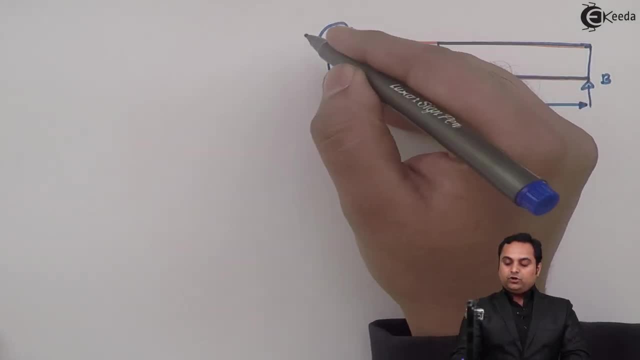 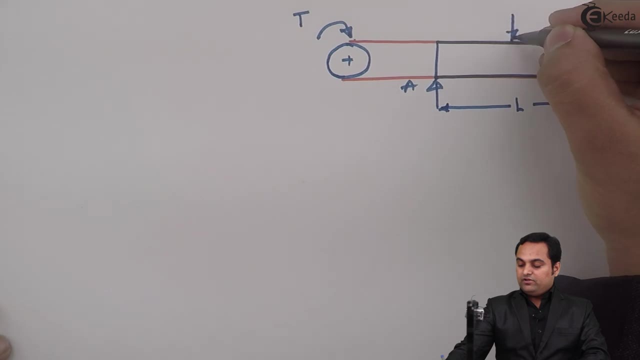 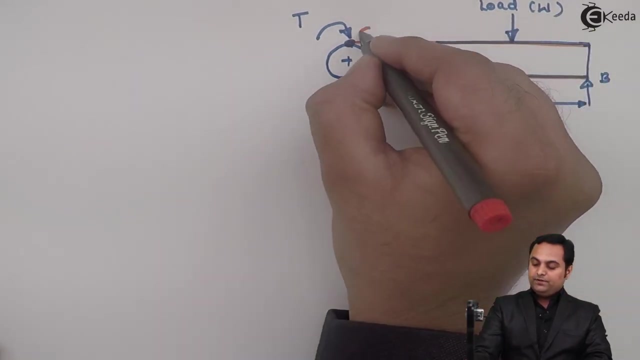 Next, The shaft is continuously rotating. torque is provided to this shaft so that it can continuously rotate. Now, if we have a load which is placed over this shaft, then because of this load, what will happen is here. I will say that this top point is point C and the bottom point 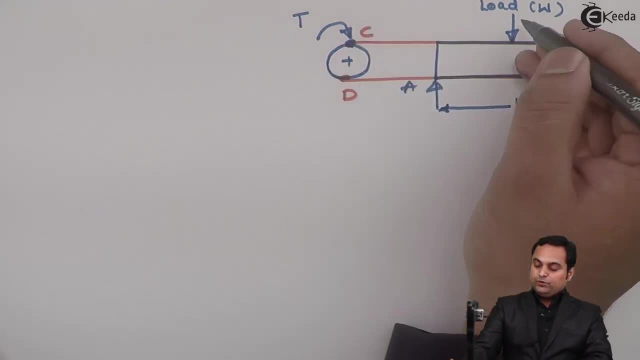 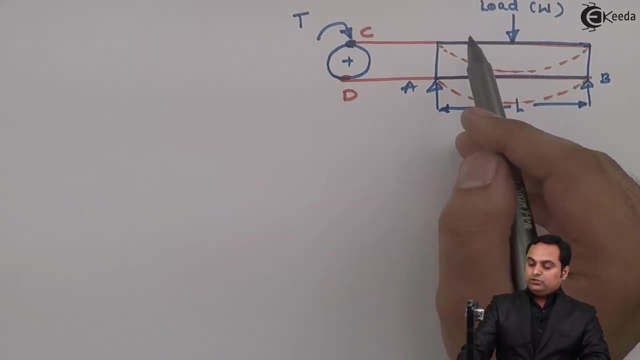 is point D, Now the load is kept on point C, So when the shaft is rotating, at the same time the load is acting. then this shaft will bend. It will bend in this form, That is, the top layers would be in compression and the bottom layers in tension. 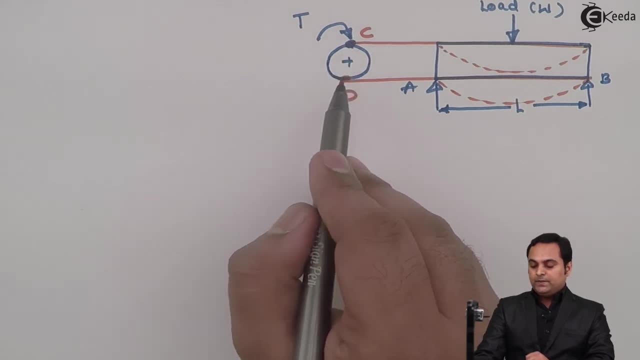 So at point C it will be in compression, At point D it will be in tension. Next, When the shaft is rotating, and then point D takes the position of point C, That is, in the next cycle point D will be at the top. 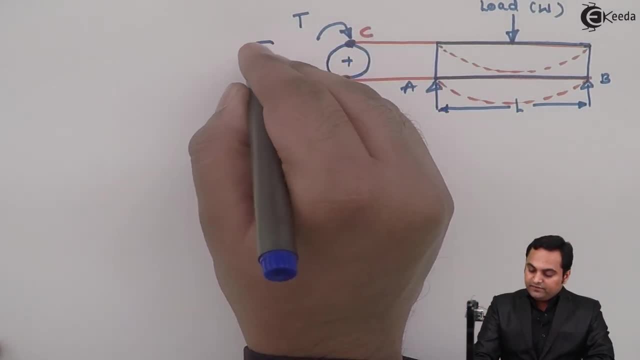 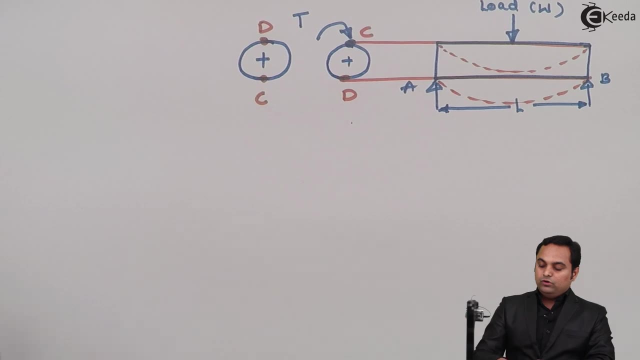 When the shaft is rotating. in the next cycle here point D will be at the top and point C will go at the bottom. because of continuous torque or continuous rotation, given Now, point D will be subjected to compression and C will be subjected to tension. and again, 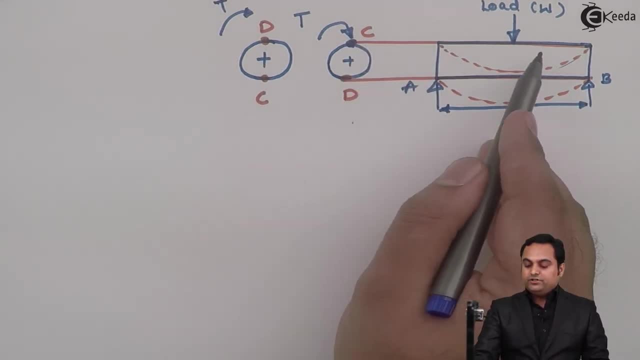 when the cycle gets repeated, then C will be again the same. So this is the point C. After this, point C and point D will be subjected to compression and point D will be the same. Then C will be again subjected to compression and D will be tensioned. 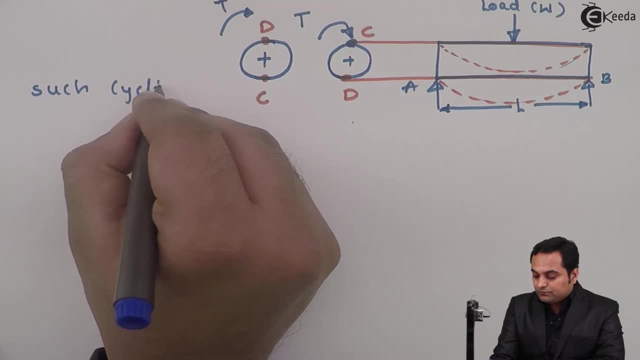 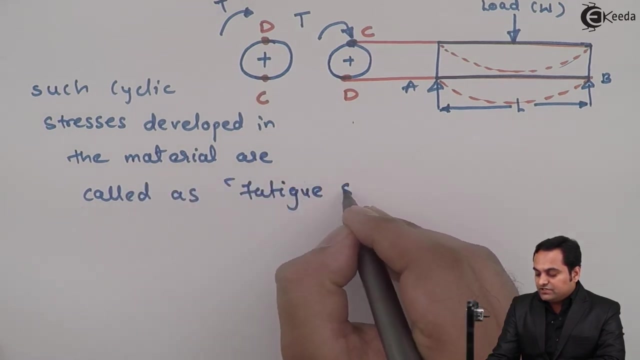 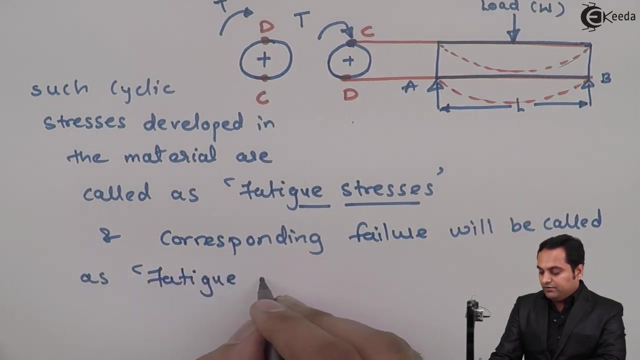 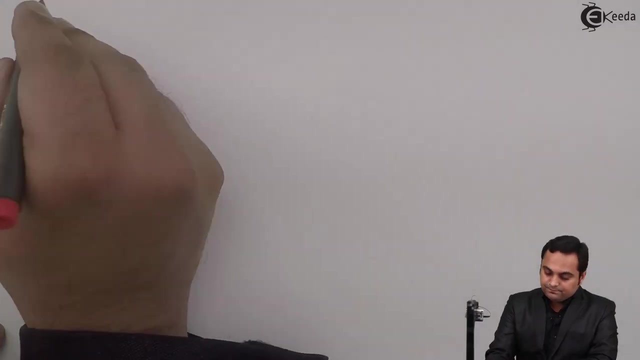 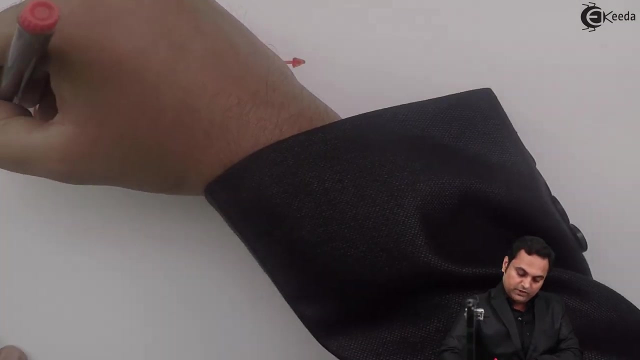 So such cyclic stresses developed in the material are called as fatigue stresses and be called as fatigue failure. and hence this shaft will fail at a stress value which is less than the maximum stress, and then that would be called as the fatigue failure. Next, here I will draw some graphs on y axis. here I am having stress. on x axis, here we 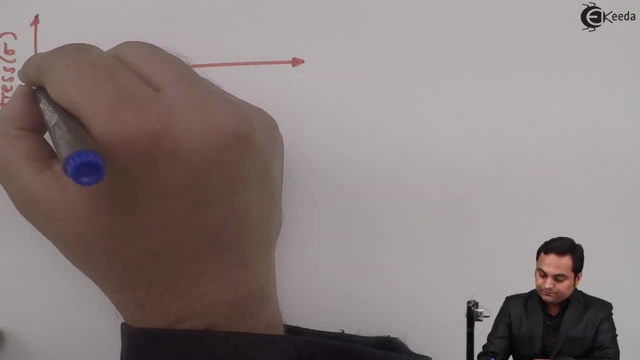 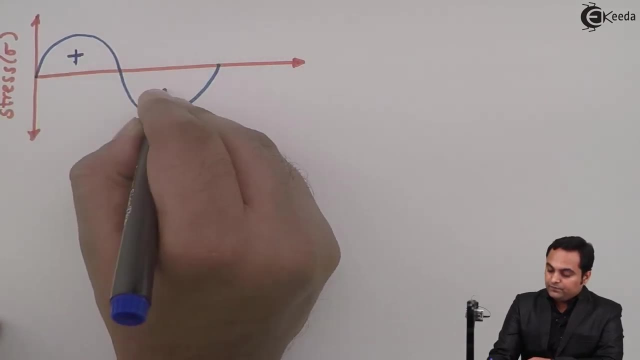 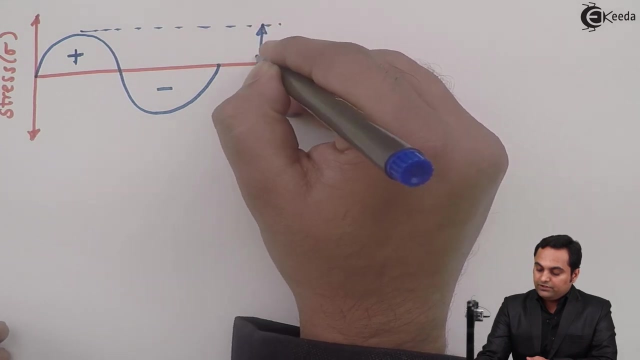 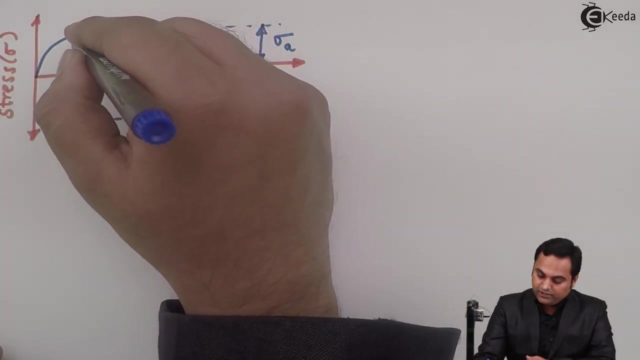 have number of cycles and then I will plot it. So here there is positive and negative value And these are called as stress, Alternating stress, sigma a. similarly, here also we have alternating stress, sigma a, and with respect to the reference up to the top, we have sigma r, that is the range of stress. 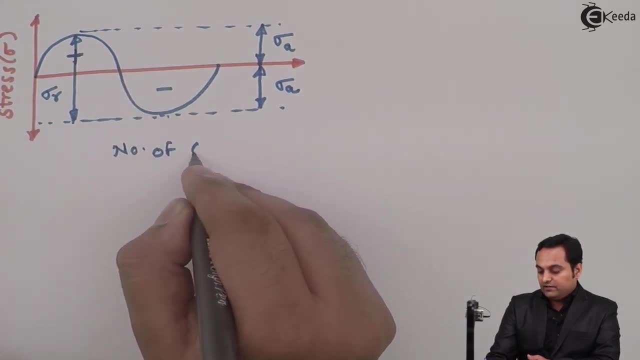 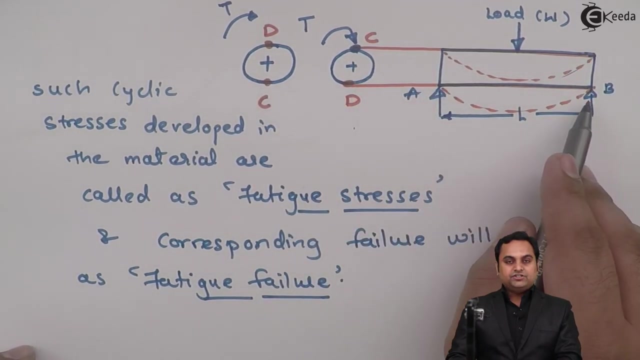 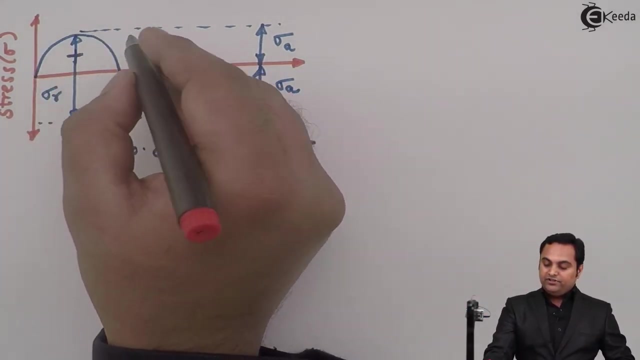 and on x axis we have number of cycles. So this example Is similar to the example which I have given, that there is a shaft which is subjected to continuous compression and tension and the cycle is going on, repeated. So we have the stresses as first: positive positive means, tensile negative stresses. 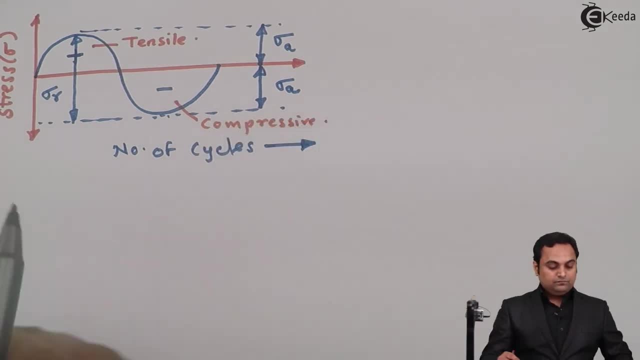 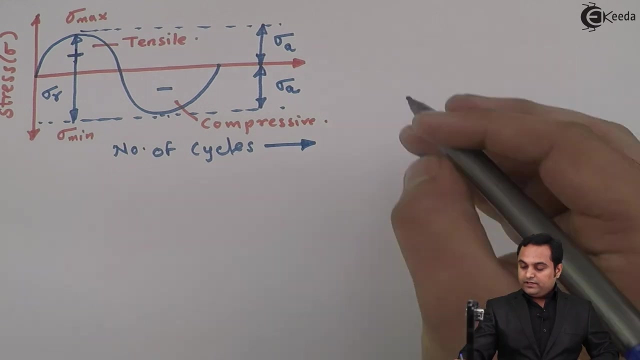 means compressive. So here I can say that, Therefore, The reference which I am taking here, this will be the minimum stress from where I am measuring sigma r and this is the maximum stress which I am getting. So therefore, here I can say that sigma r, that is the resultant stress, will be sigma max. 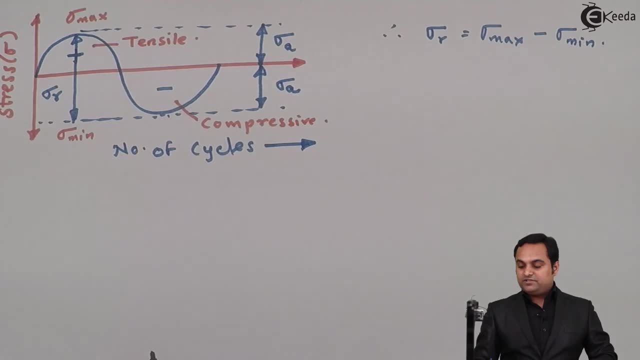 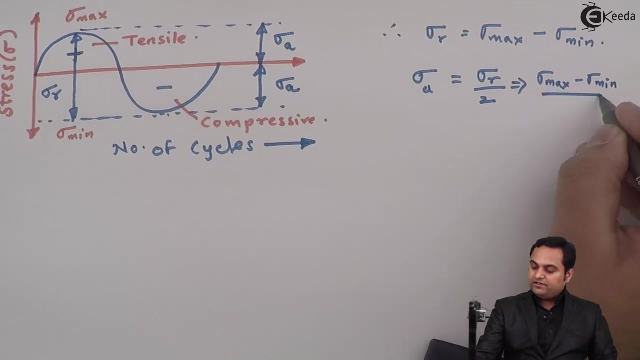 minus sigma min, it is sigma max minus sigma min. Next, sigma a, that is the alternating stress, will be sigma r divided by 2.. So now, here I have written the alternating stress, sigma a is equal to half of sigma r. So therefore, sigma r is sigma max minus sigma min, divided by 2.. 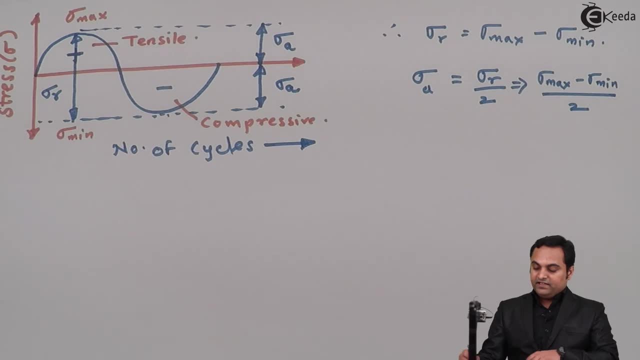 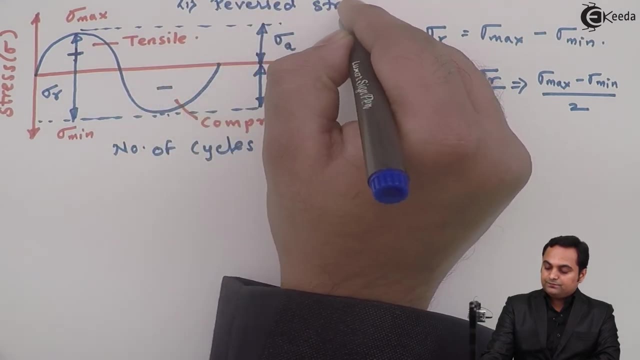 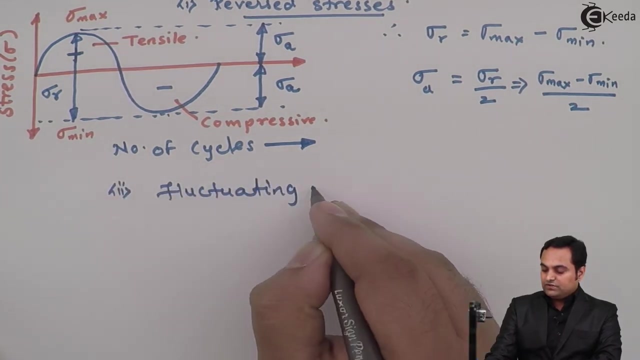 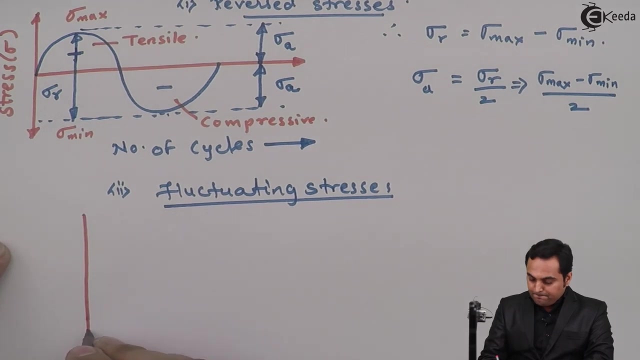 So this is the alternating stress and this complete diagram which I have drawn. it is for. it is also called as for reverse stresses. Next, I will draw a diagram For fluctuating stress. Next, I will draw a diagram For fluctuating stresses: Stress versus the number of cycles. 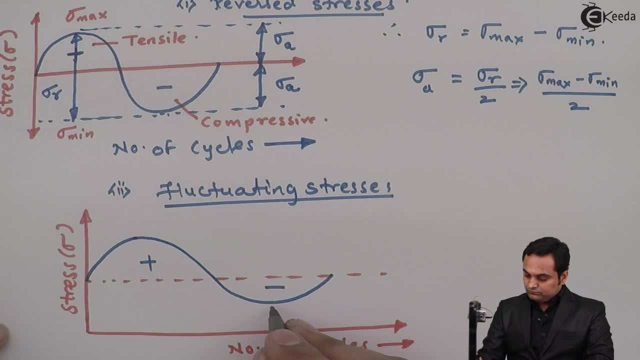 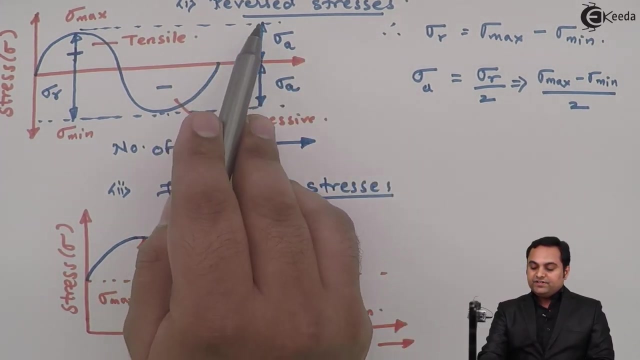 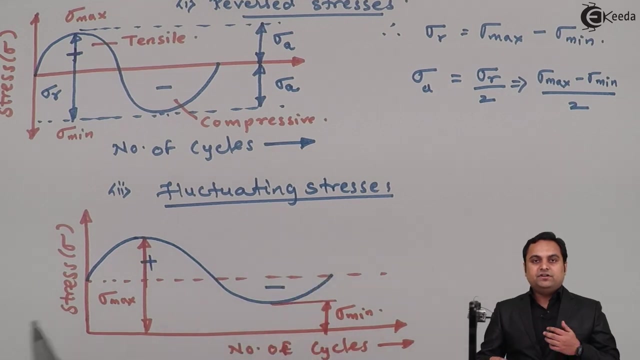 Now, previously we have seen, in case of reverse stresses, the alternating stress, that is, the stress in tensile and compressive nature, They were having the same value. But in the case of fluctuating stresses the values may differ. that's first, as we are. 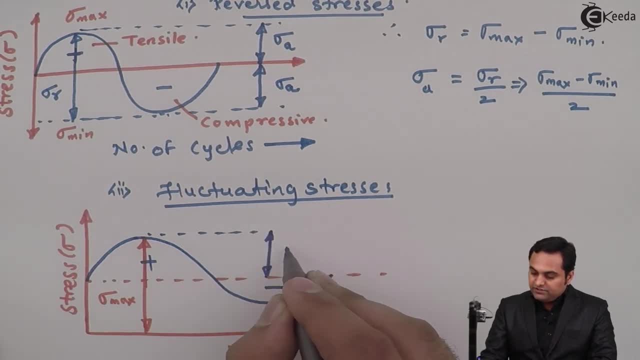 seeing here, this much is the tensile stress value and the remaining this much is the compressive stress value. as we can see, the stresses values are different now from this. i can say that therefore, we can plot the mean stress out of this, the mean stress. it can be written as sigma max. 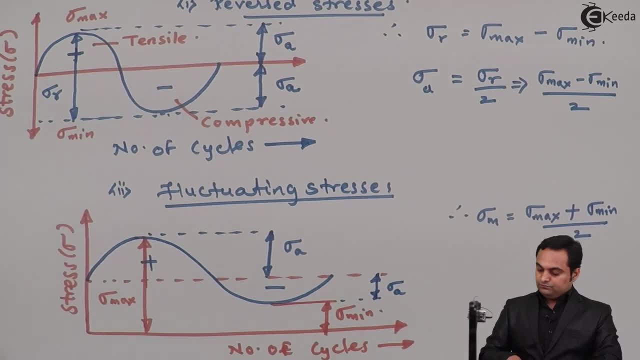 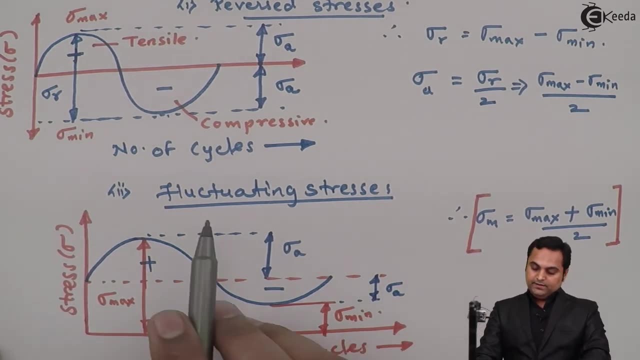 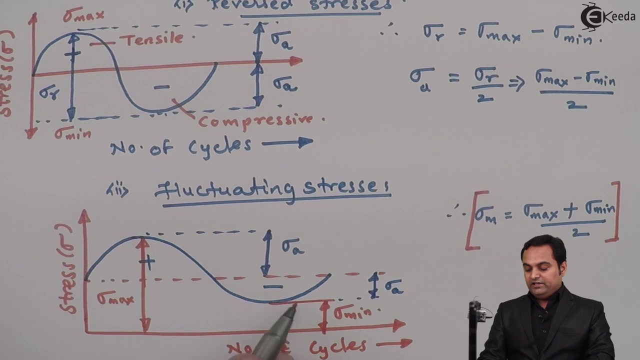 plus sigma min divided by 2. so here we can see that in case of fluctuating stresses, the stress value will go on changing, that is, from positive to negative. the values will be different, not only the nature, the values will also be different, and for that we can write the mean stress which i have written here and apart. 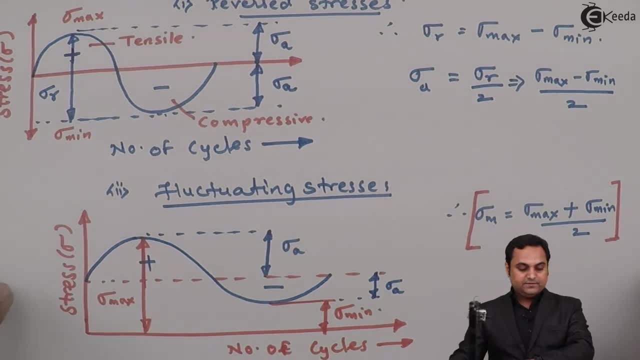 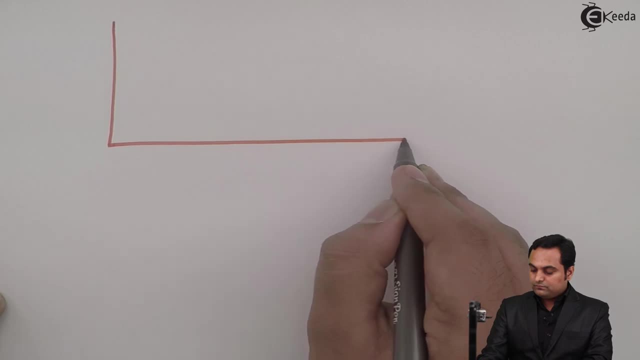 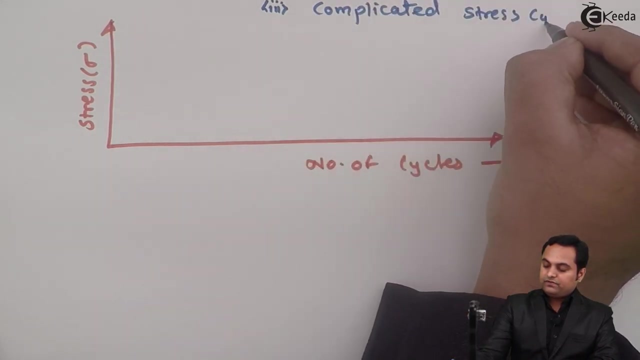 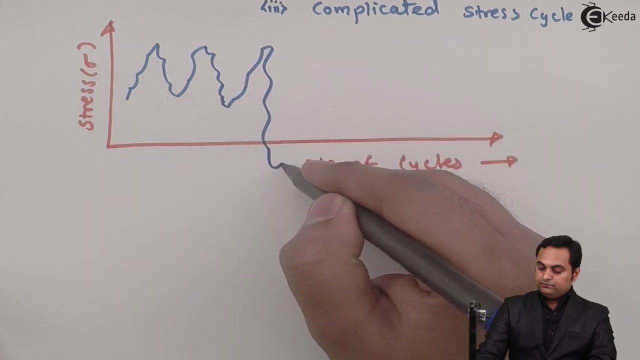 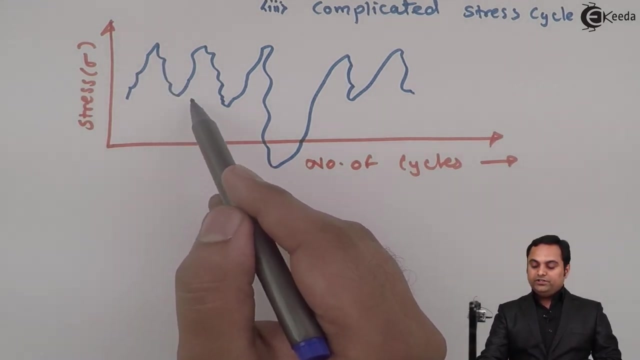 from that. this was fluctuating stresses. the next thing is you. it is a complicated stress cycle. this is a complicated stress cycle and here the nature will be wavered, that is, it won't be following a continuous path. so in case of complicated stress cycle, the stress would go on increasing and it will decrease in a 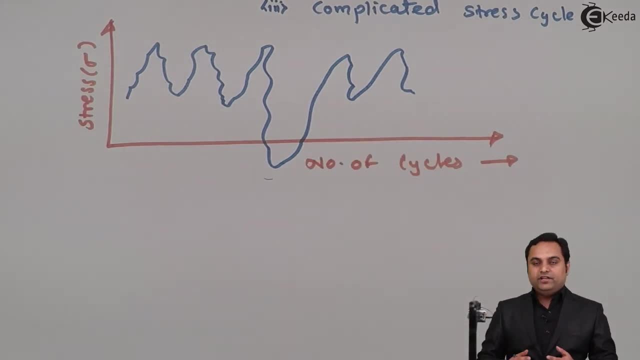 wavered manner, that is, we cannot solve it by using any of the formula. so this is the complicated stress cycle and mostly aircraft wings. they are subjected to the complicated stress cycle. so in this video we have seen what is meant by fatigue failure and we have 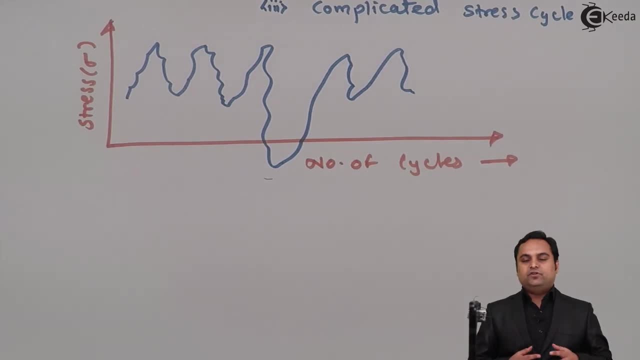 seen various graphs related to the stress and number of cycles.